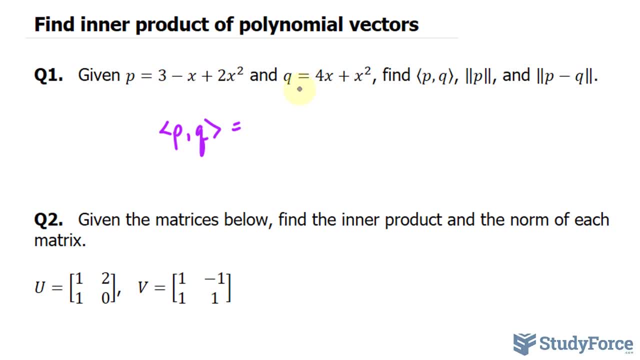 that's the term that does not have a variable, and in this expression a constant term doesn't exist. so we multiply three times zero. For the next one we have negative one. so I will add the product of negative one times four plus the coefficient of x to the power of two is two multiply. 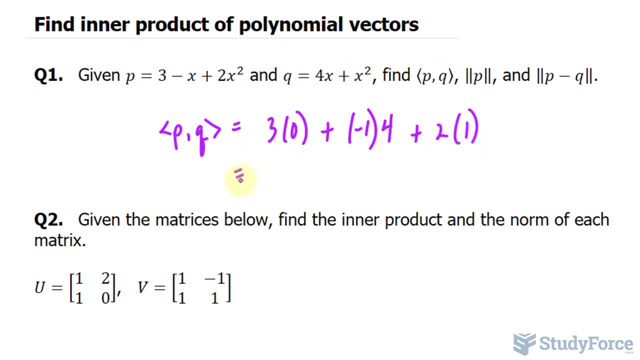 to the coefficient here, which is one. Three times zero is zero negative. one times four is negative four, and two times one is two. Therefore our answer, the inner product, is negative two. Now let's go on and find the norm of p. So to find the norm of p, let me just write this down: 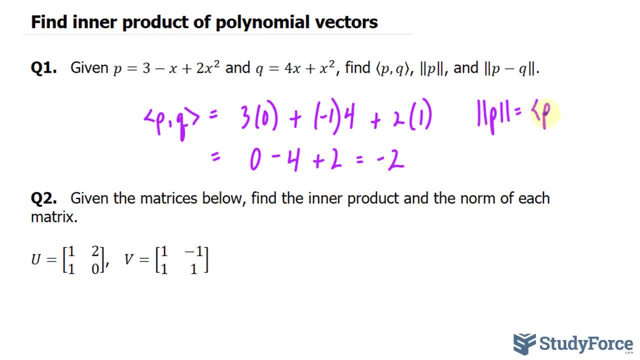 for you, it's the same thing as finding the inner product of p and p raised to the power of half, which means that we'll be doing the exact same thing, and then, whatever our answer is, we square root it. I hope I didn't lose you there, so here we go. 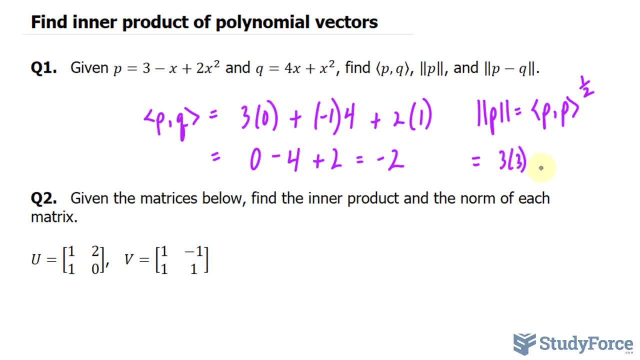 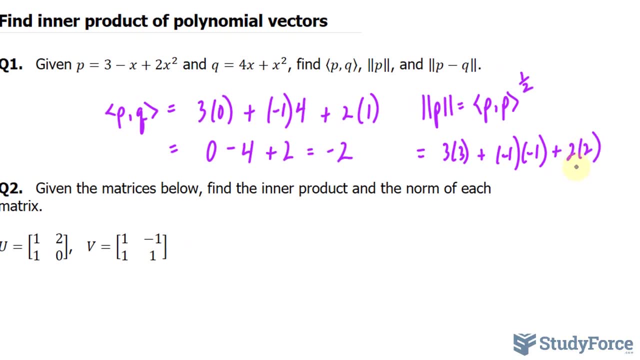 We will take three. multiply it to three plus negative one. multiply to negative one plus two times two. Whatever this answer is, we will square root it, which is the same thing as raising it to the power of half. We have nine plus one plus four. that's equal to the square root. 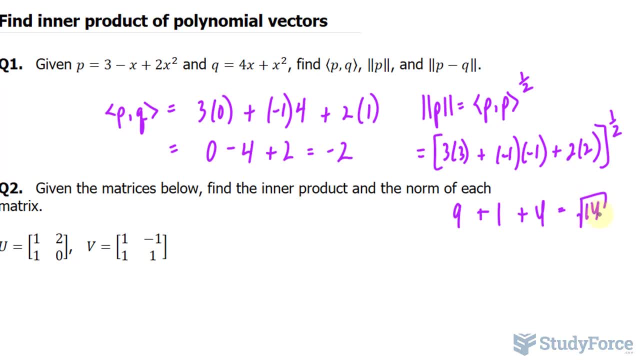 of fourteen. Now let's find the distance between p and q. To do this, we'll be subtracting each of the similar terms from both of these polynomials. So we had three, and the like term for this expression is zero. Three minus zero is three. Essentially, we are creating a new polynomial. 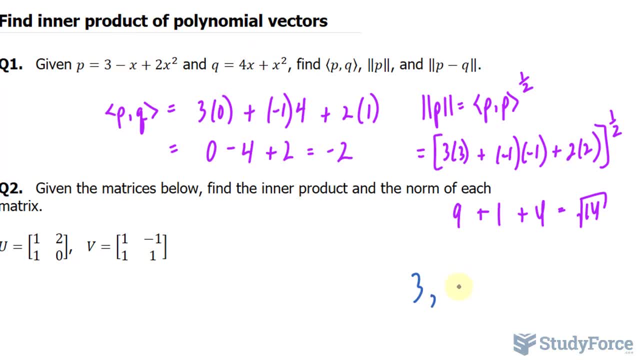 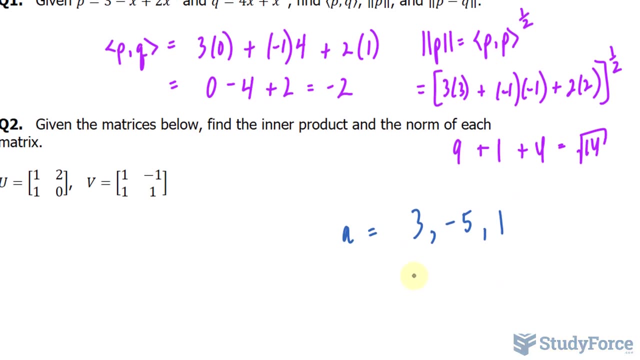 by subtracting each Negative one minus four is negative five, and two minus one is one. So we can call this polynomial anything we like. Let's just call it a, and it has these three terms. Think of a as being three minus five x. 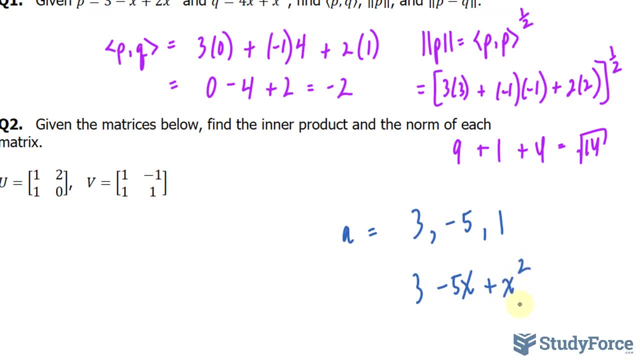 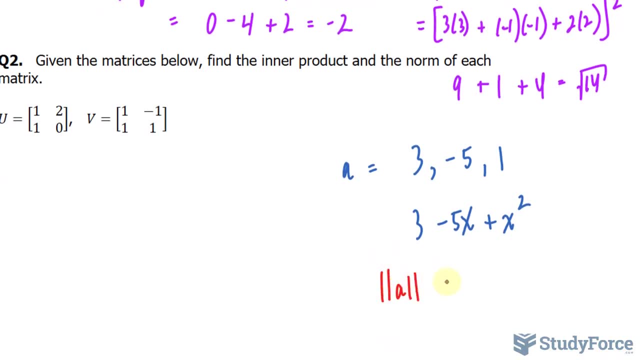 plus x, the power of two. And now we find the norm of this, the same way we did up here with p, So I'm going to find the norm of a, and we end up with the square root of three times three, or three squared negative five. 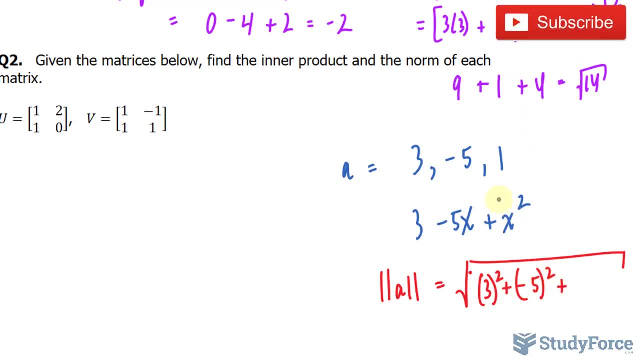 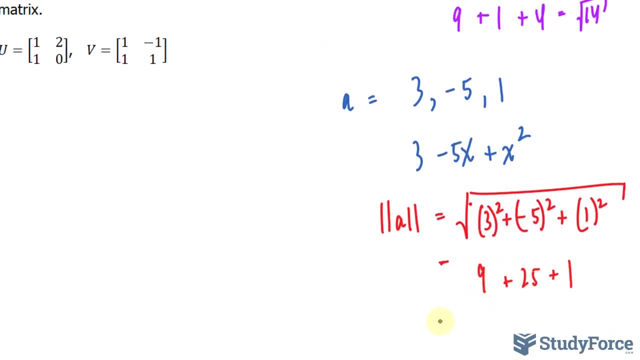 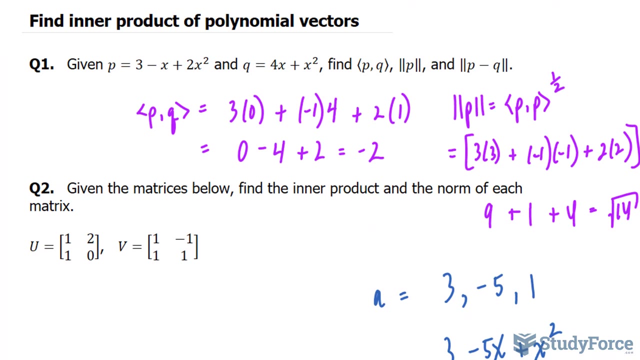 raised to the power of two plus one raised to the power of two, We should end up with nine plus twenty-five plus one. Twenty-six plus nine is thirty-five Square root of thirty-five. that's the answer to question number one. Now I know this. 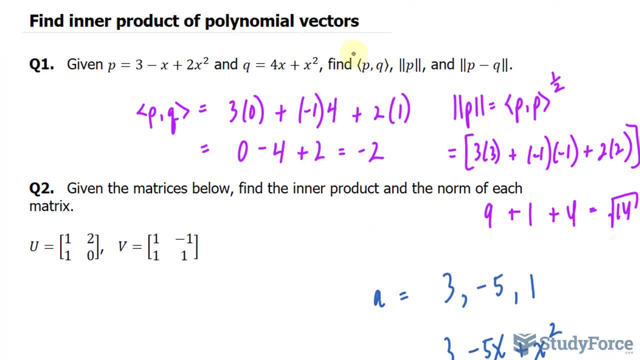 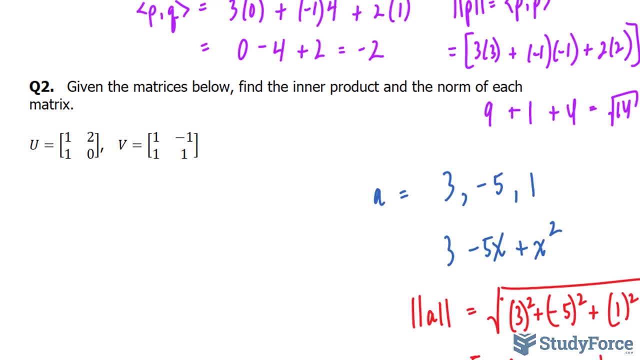 video talks about polynomial vectors, but I just wanted to throw in a matrix one. We're asked, given the matrices below, find the inner product and norm of each matrix. So the first question caters to polynomials. This one caters. 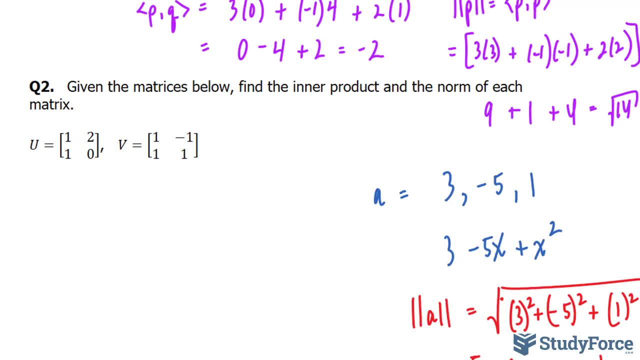 to matrices What we do in this situation. if we want to find the inner product of a vector, u and v, we will multiply each element in their respective location together. So I'll multiply 1 and 1, this element and this element together, plus 2 and negative 1, plus this one and that one. 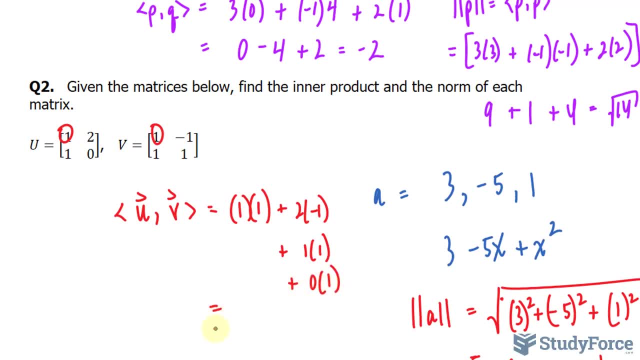 plus 0 and 1.. 1 plus negative, 2 plus 1, that's equal to 0.. Now to find the norm of u. it's like doing the same thing as this, except we now have both u's, So pretend that both of. 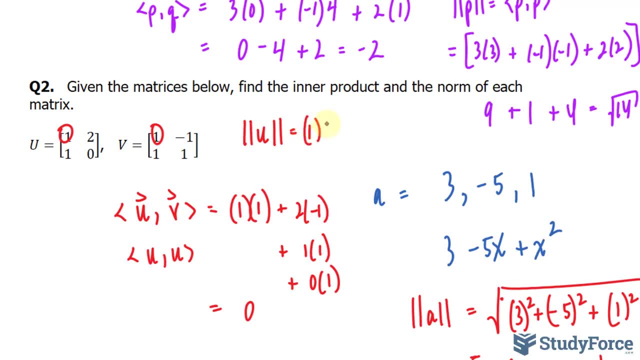 the matrices are the same. we have 1 times 1, plus 2 times 2, plus 1 times 2, plus 1 times 2, times 1, plus 0 times 0.. 1 plus 4 plus 1 is 6.. And of course, don't forget, just like how we did. 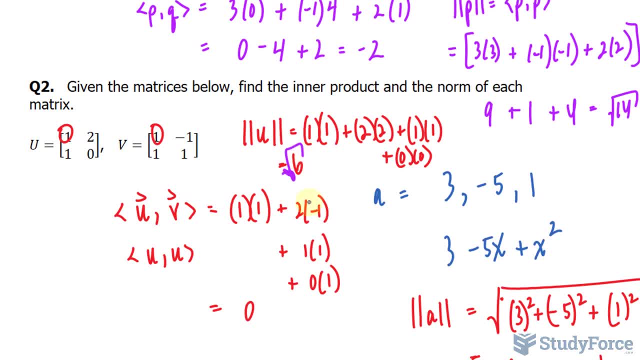 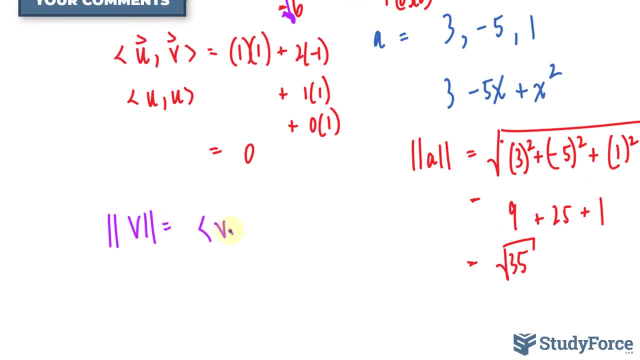 in question number 1, we will square root this. Let's do this one more time for v. So let me write it out like this: That's the same thing as the inner product of v and v raised to the power of 1.. 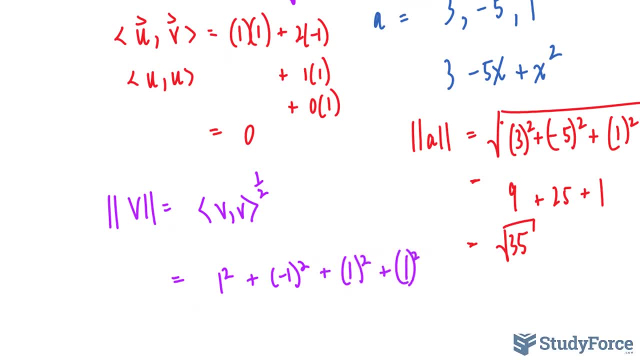 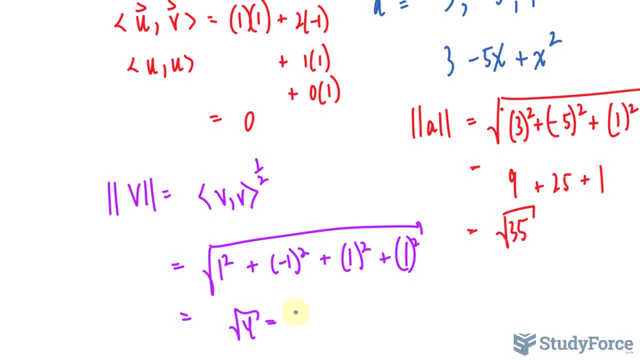 1 squared plus again 1 squared. We will now raise this or square root it. We get 1s across. the square root of 4 is 2.. And there you have it, a quick video on how to find the inner product.